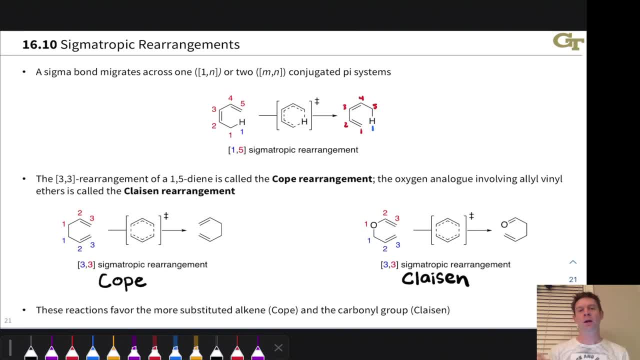 rearrangement like a 1,5 or a 1,7,. a sigma bond appears to migrate over one pi system, with the other end of the sigma bond kind of just along for the ride, and this may be an atom like H or a group like CH3.. In an M-in sigmatropic rearrangement where M and N are both not equal, 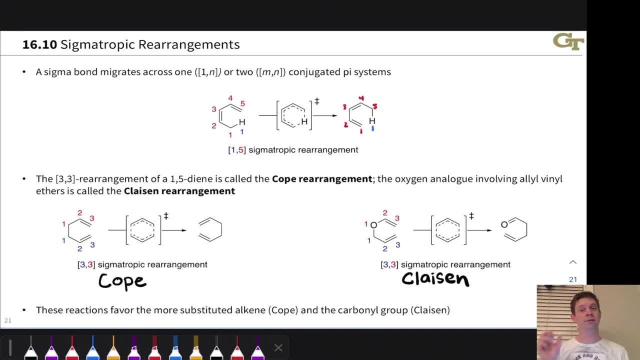 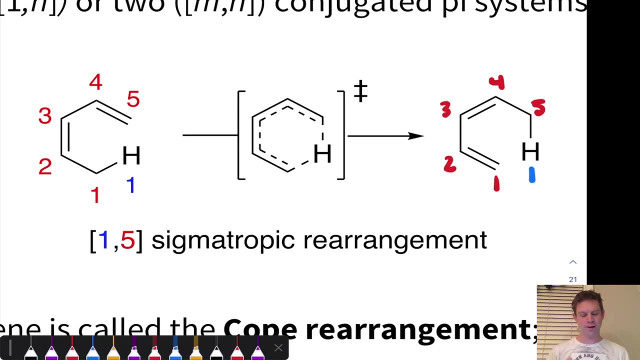 to one, then two pi systems are involved and both ends of the sigma bond appear to migrate. We'll see examples of both in this video. Let's start with an example of a one-in rearrangement, the 1,5 sigmatropic rearrangement. We zero in on this and pay attention to the bonds made and broken. 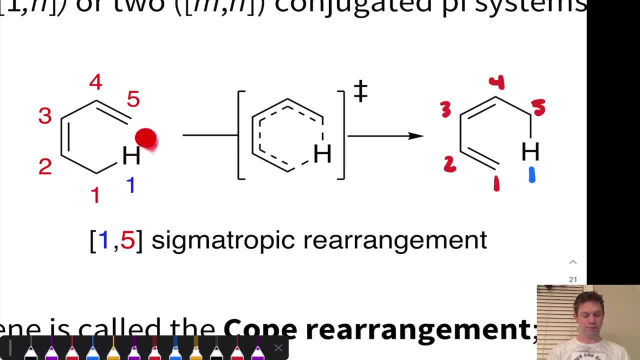 We can see that the H1C1 bond right here is broken and a new bond is made between H1 and C5. So what appears to be happening is this bond right here appears to be migrating from carbon 1 to carbon 5, and this is called a 1,5 sigmatropic rearrangement because of 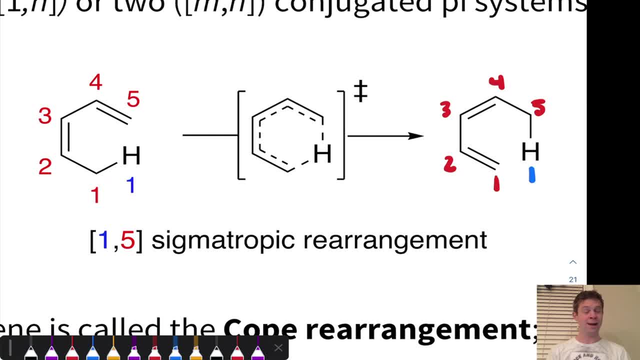 the migration along these atoms in red. that's where the 5 comes from and the fact that the other end of the sigma bond stays put attached to hydrogen 1 the whole time, and that's where this blue 1 comes from. 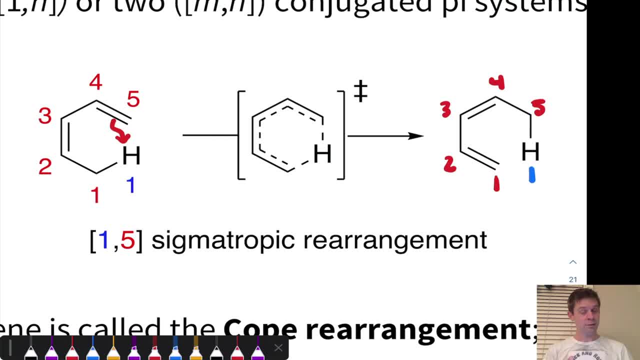 The electron flow here is cyclic. The new sigma bond is actually not the same electron pair in the original C1H1 bond, but is this pair of pi electrons between carbons 4 and 5, and electrons flow in a cyclic manner so that everything stays neutral throughout the elementary step and in the transition. 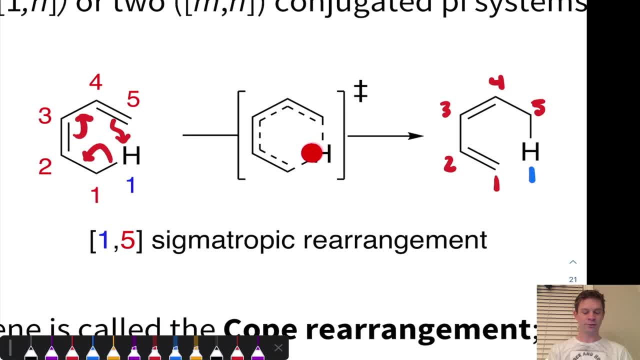 state. we've got a fully cyclic array of electrons here, including the electrons involved in the newly forming and the breaking C1H1 bond bond. So we've got a cyclic array of electrons here in the transition state and in the product we can see this migration of the CH bond from carbon 1 to carbon 5.. So this is a pretty typical 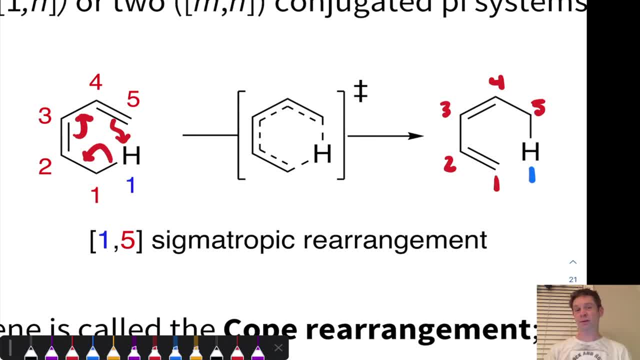 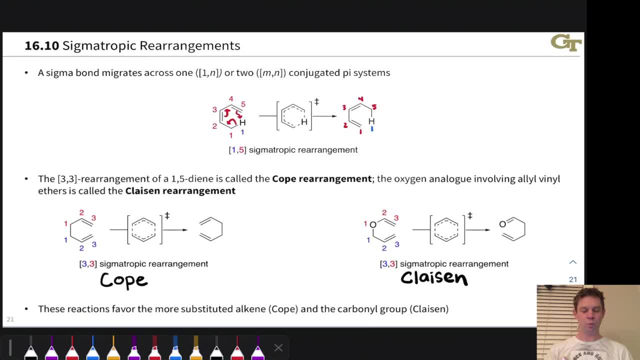 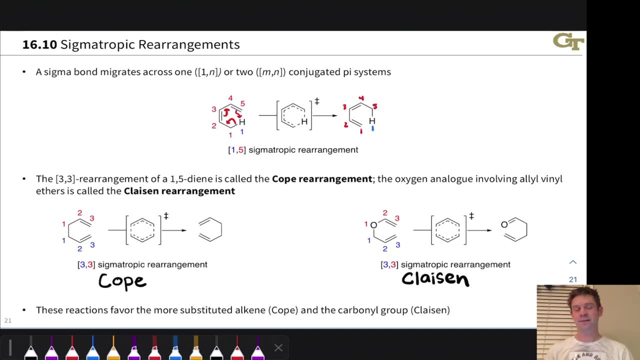 1, 5 sigmatropic rearrangement and that's pretty much all we're going to say about 1. in sigmatropic rearrangements There's a whole orbital symmetry analysis you can do for these. that is well beyond the scope of CHEM 2312.. There are two synthetically important 3, 3 sigmatropic rearrangements that 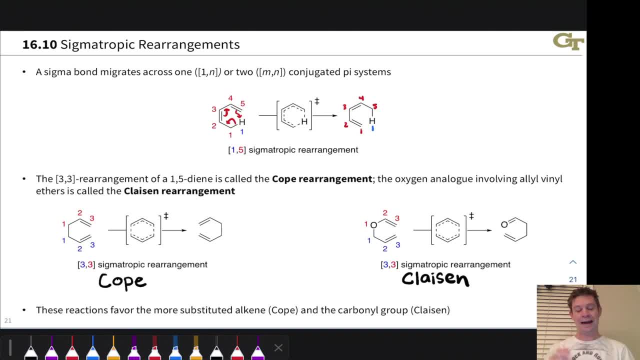 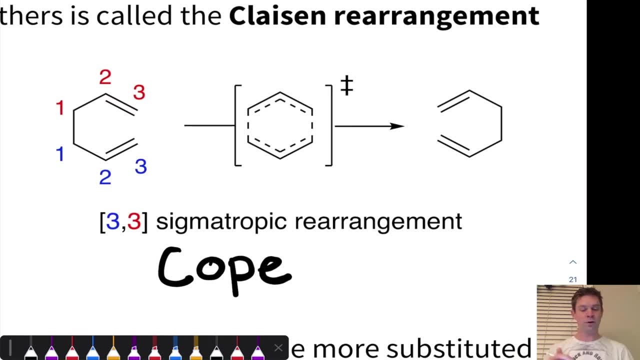 we're going to spend the rest of our time in this video on The Cope and the Claisen rearrangements. The Cope rearrangement is kind of the classic 3, 3 rearrangement and it involves substrates that are 1, 5 dienes, Dye, alkenes, with a single bond or three single bonds between the. 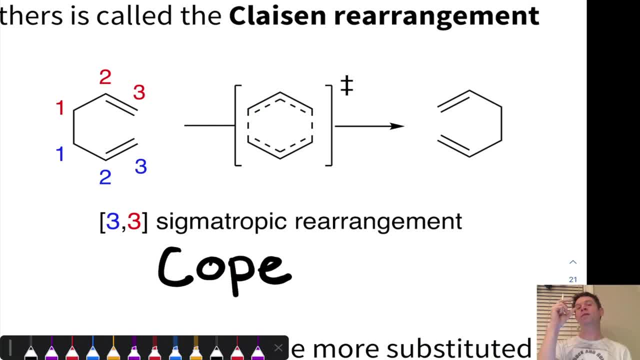 alkenes With the migrating sigma bond, that one that's in the middle. So we have here an alkene. You can think of this as bond 1.. Here's bond 2,, 3,, 4, and 5.. This is a 1, 5 diene and this is the prototypical. 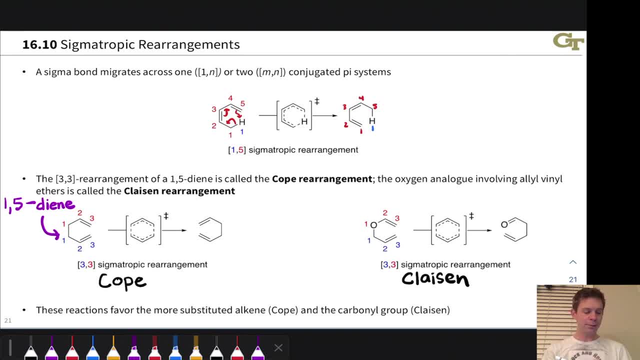 substrate for the Cope rearrangement. The migrating sigma bond is between the carbon 1 in red and the carbon 3 in blue, And that's right here. So the migrating sigma bond appears to have walked three steps from carbon 1, 2, 3 on the red side and three steps on the blue side: Carbon 1, 2, 3.. 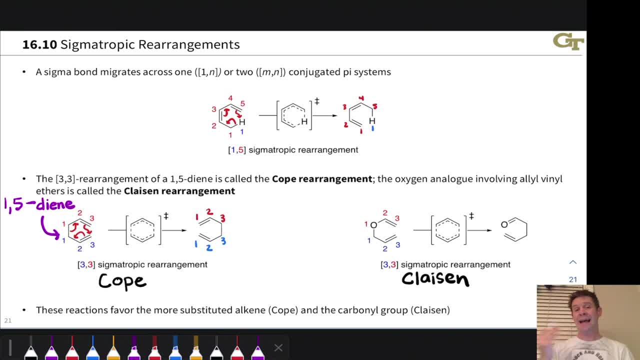 That's why this is called a 3, 3 sigmatropic rearrangement And, as in the 1, 5, in the transition state we've got a fully cyclic array of electrons, including the electrons and the electrons involved in the forming and breaking sigma bonds. This is called the Cope. 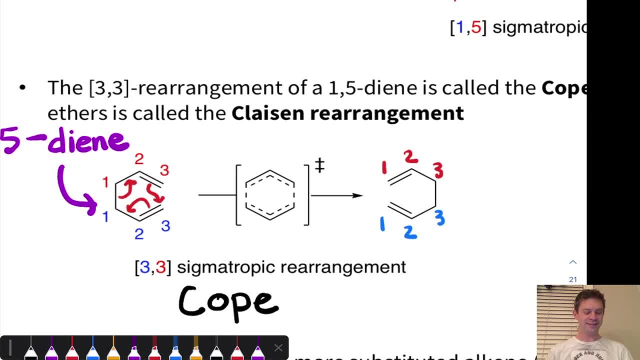 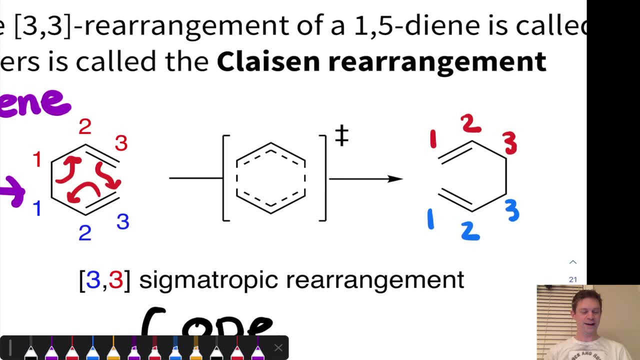 rearrangement. Now, in this case the product is identical to the starting material, And that's worth pointing out. right, These are both 1, 5 dienes. They have the exact same structure, They are identical molecules, And so this rearrangement is entirely reversible, as shown here In. 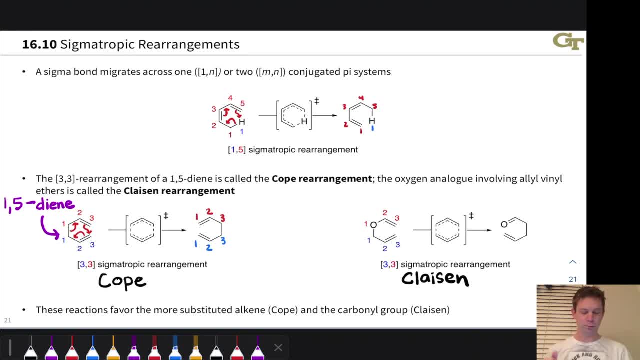 synthetically useful Cope rearrangements. there's some kind of driving force And we'll return to that in a second. The oxygen analog of the Cope rearrangement, where we've got the oxygen analog and we replace one of the carbons in the saturated chain here with an oxygen, is known as the. 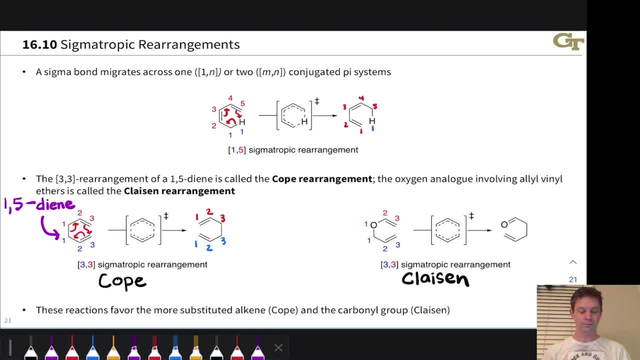 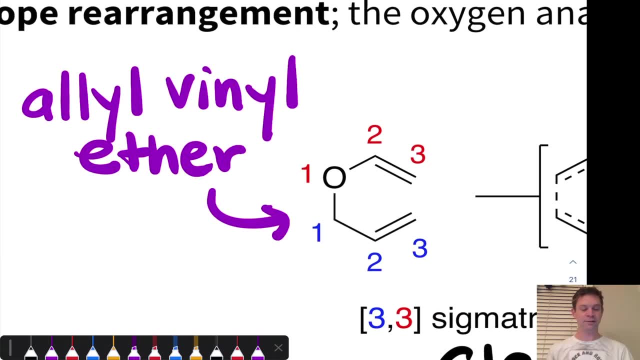 Claisen rearrangement, And the Claisen has a built-in driving force. The prototypical substrate for a Claisen rearrangement is an allo-vinyl ether, And you see pretty much the simplest example of this type of compound right here: Allo-vinyl ether. we have a vinyl group As it's. 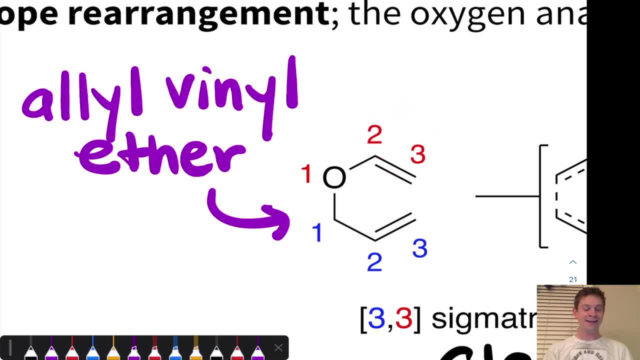 labeled. here it's carbons 2 and 3, part of the vinyl group and an allo group, And here that's carbons 1, 2, and 3. in blue is an allo group. So it's an allo-vinyl ether And if you think about this, this is a very similar structural 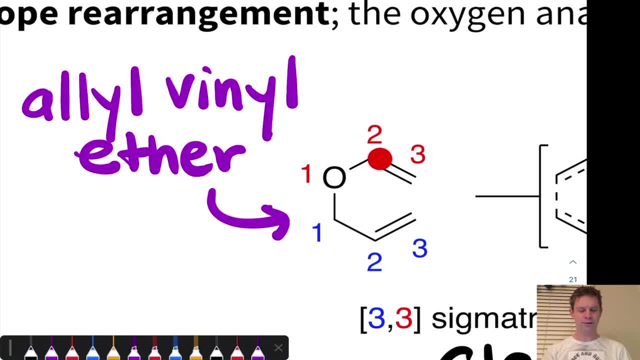 pattern to the 1, 5 diene of the Cope substrate. I've got a double bond. Here's bond 2, 3,, 4, and 5.. So this is a 1, 5 diene that just happens to have an oxygen in the middle, And these can. 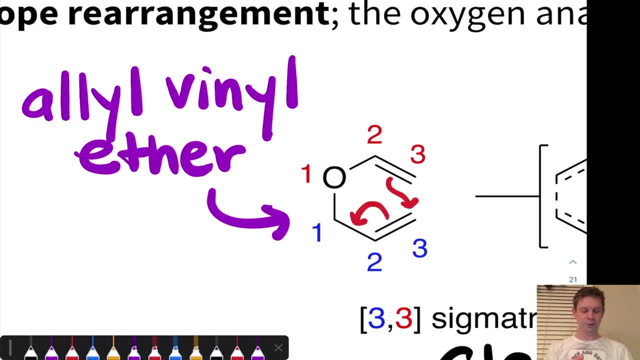 rearrange via electron flow. that is exactly analogous to the Cope situation: cyclic electron flow like this, And it's a 3, 3 rearrangement. The bond between carbon- 1 in blue- and oxygen- 1 in red- appears to migrate to the three positions on both fragments: the O, C, C in red up here. 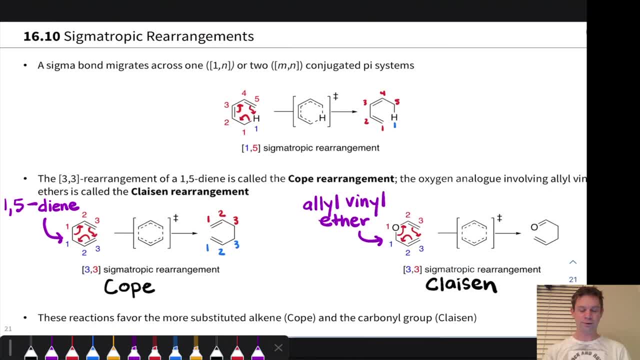 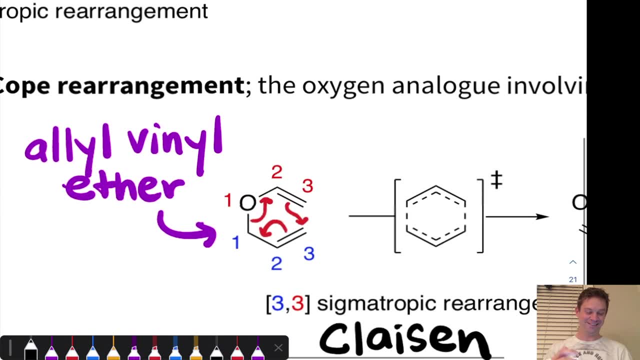 and then C, C, C in blue at the bottom. So this is a 3,- 3 sigmatropic rearrangement. Actually, I'm just noticing now that the transition state needs an oxygen in it right. This is very similar to the Cope transition state. It's just going to have an oxygen right there as opposed to 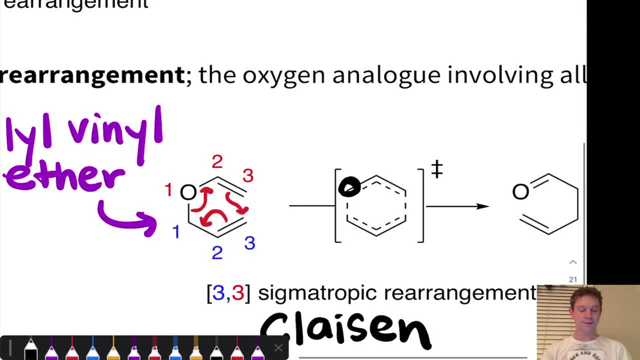 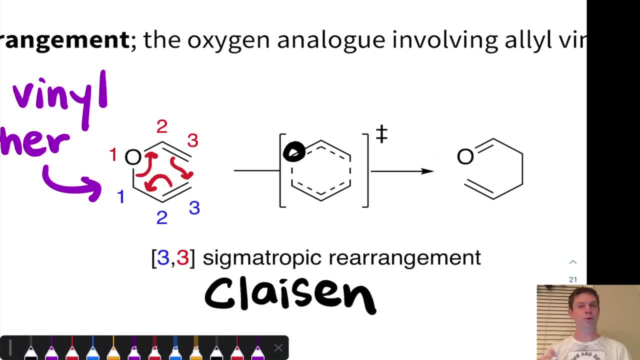 a carbon or a CH2 group And the product of the Claisen rearrangement notice contains a carbonyl group, contains a CO double bond, And this is an important distinction from the Cope rearrangement. That CO double bond provides a built-in driving force for a lot of Claisen. 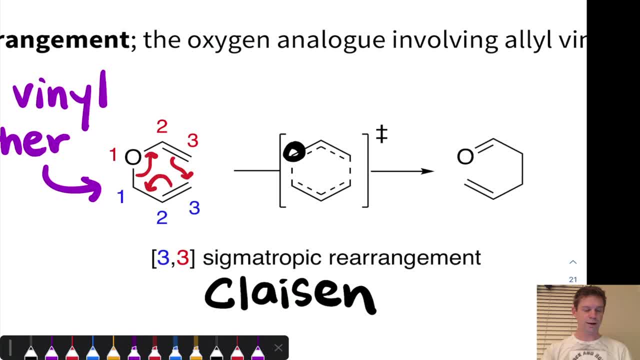 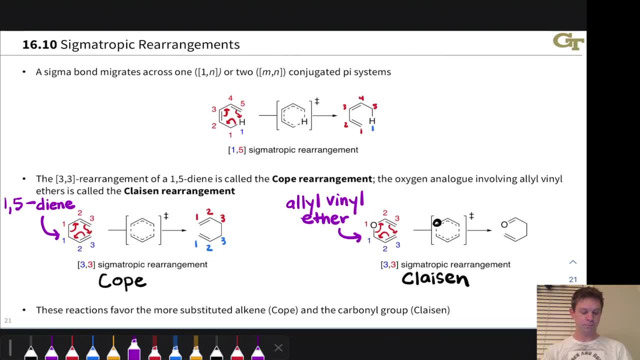 rearrangements, since the CO double bond is quite strong and quite stable. So, although these reactions are often reversible, these 3, 3s, particularly in the case of the Cope rearrangement, when we're forming a more substituted alkene- in the case of the Cope rearrangement- or relieving 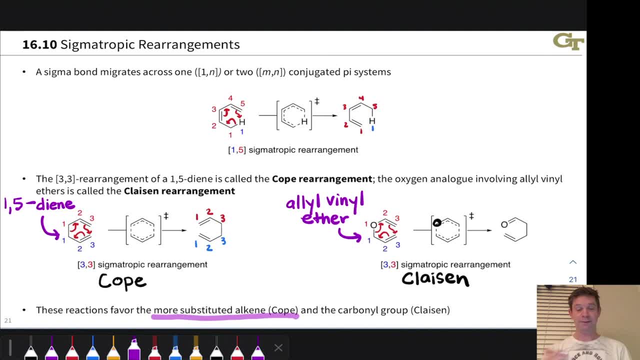 some kind of strain. that will often favor the products And in the case of the Claisen we've got that built-in driving force of the carbonyl group forming in the product. Allo vinyl ethers will often spontaneously rearrange to form these products in which we got CO double bonds. 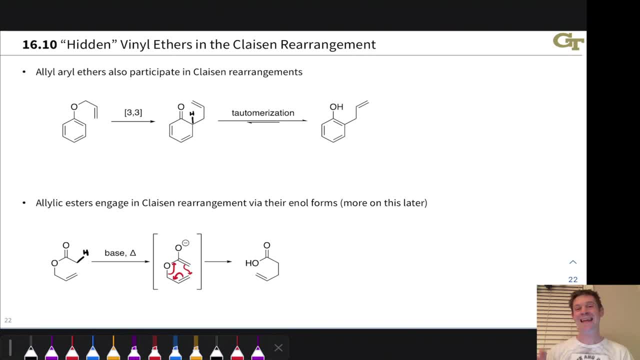 Finally, I just can't help but mention a couple of circumstances where some hidden vinyl ethers show up in Claisen rearrangements, And the first case here involves not an allo vinyl ether but an alloaryl ether And an alloaryl ether. 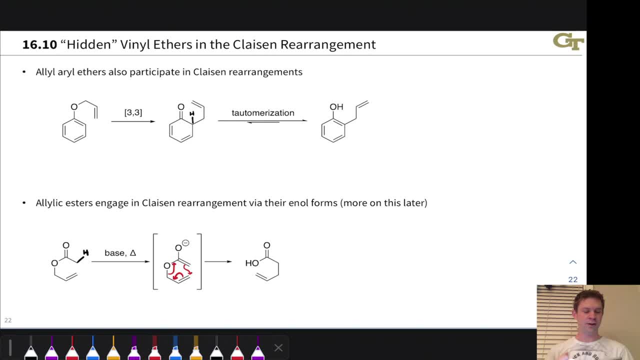 there is a double bond in the right position. engage in a Claisen rearrangement. Another way of saying this is: this is kind of a 1,5-Dione, right, We have a alkene right here. Here's bond 2,, 3,, 4, and 5. It's a 1,5-Dione, so it can do. 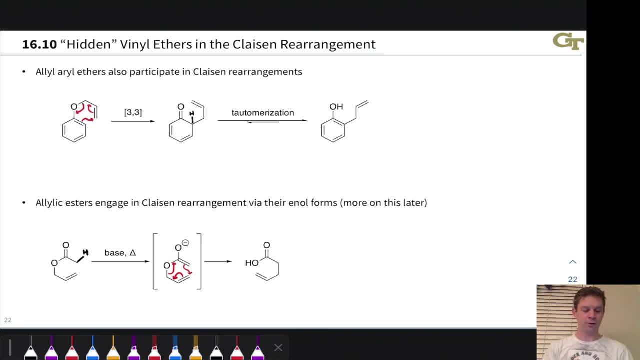 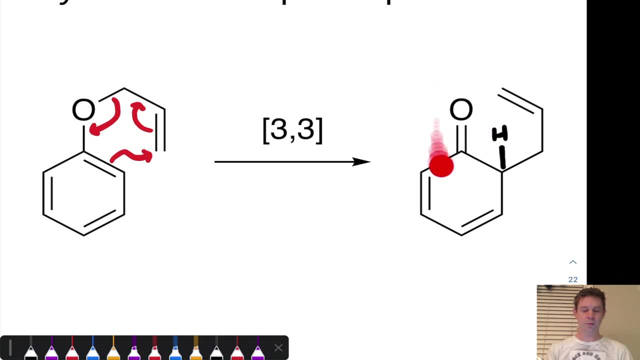 3,3-sigmatropic rearrangement through electron flow. that looks like this, And if we zoom in here, the product that forms initially is this carbonyl-containing product. Now, for reasons we'll explore later, after we've talked in more detail about carbonyl compounds, 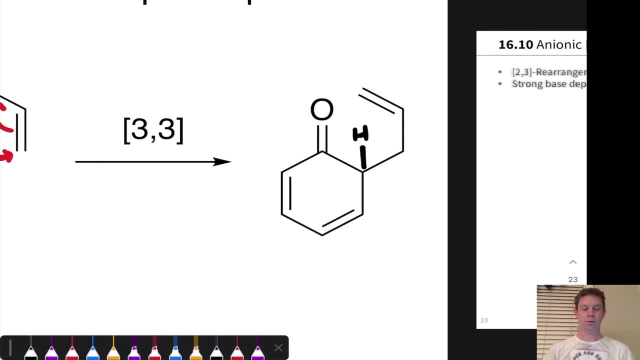 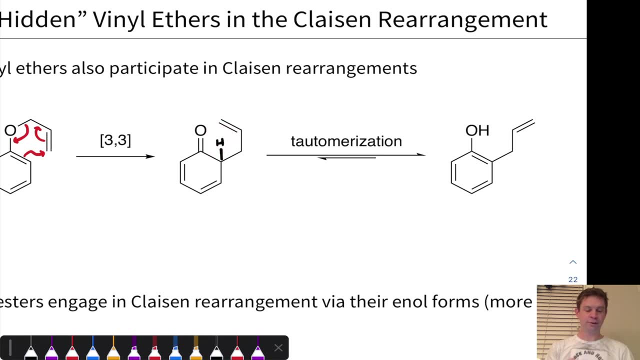 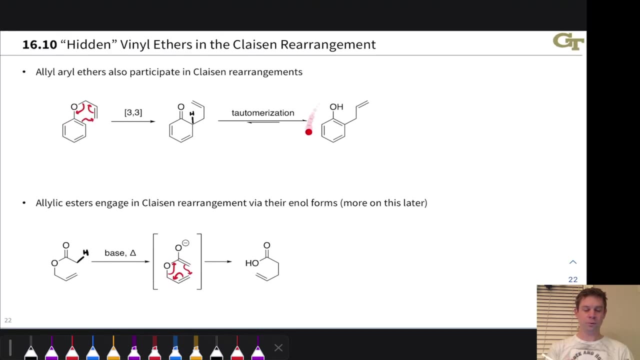 this is going to spontaneously react to form an isomer in which this hydrogen that we've drawn out explicitly migrates to this oxygen and a double bond shifts over. And this occurs because the product that we form ultimately here is aromatic. So there's a big driving force to 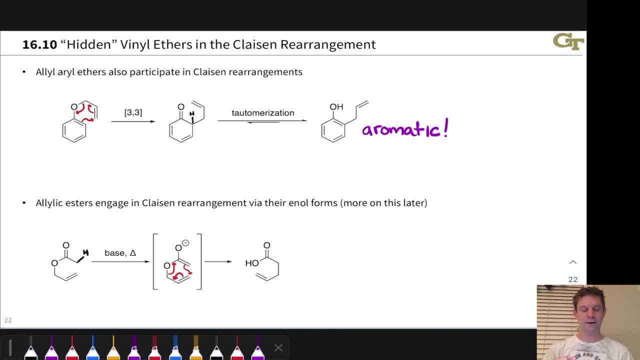 reestablish aromaticity after the Claisen rearrangement has taken place. These two compounds are isomers. They're known as tautomers, and we're going to talk a lot more about tautomerization. We're going to talk a lot more about this later in the course, so stay tuned. 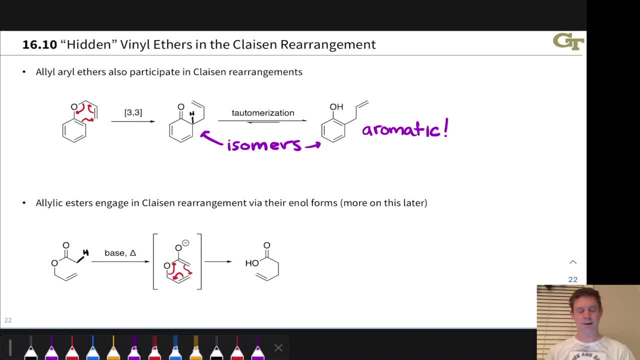 Another place where a hidden vinyl ether comes up is when we create a new double bond through deprotonation and the creation of what's called an enolate. So I want you to imagine a base coming in and deprotonating at this position. We'll talk about why this position is rather acidic. 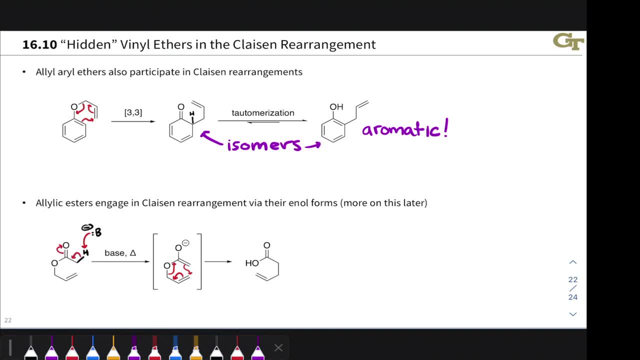 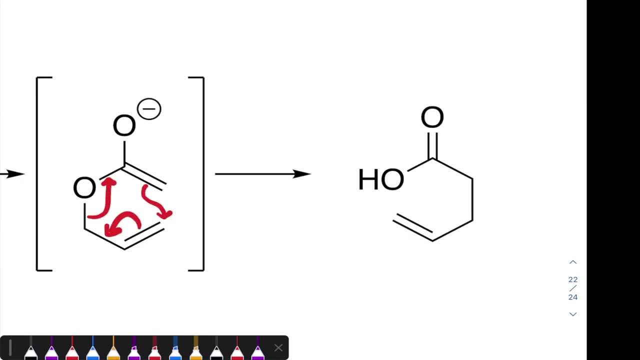 later in the course, but for the time being, take my word for it that this deprotonation can occur with a reasonably strong base, And then we get a structure that looks like this: Now, this is a 1-5 diene: 1, there's a 5 key in there: 2,, 3,, 4, and 5. And so it can engage in Claisen. 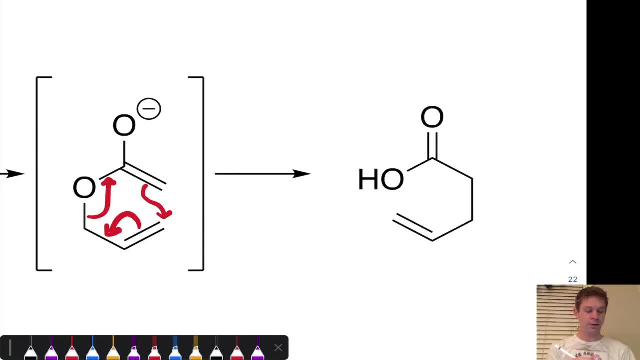 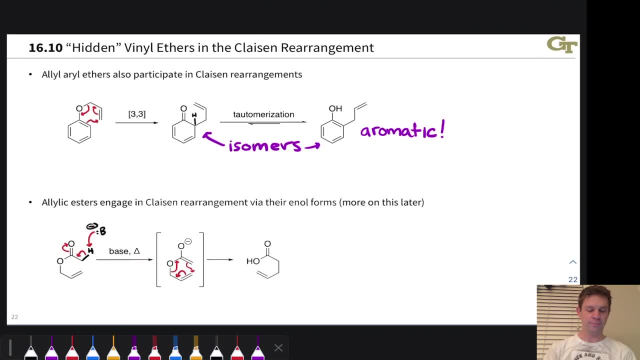 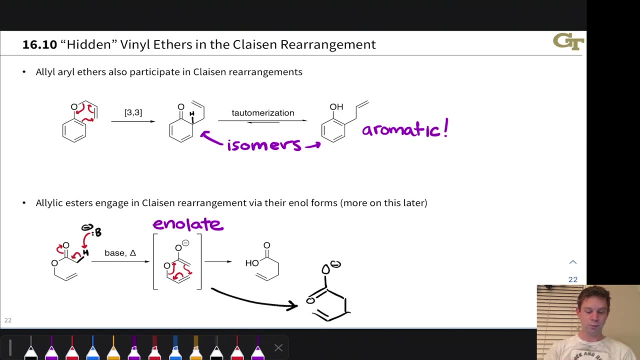 rearrangement, And when it does this, we go from a C-C double bond and a C-C double bond to a new C-O double bond. So there's a driving force there. Now you may notice that the final product drawn here is neutral, and this is because initially, we end up with an anion and that anion. 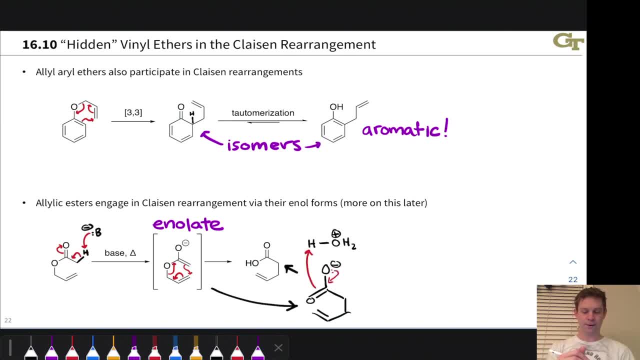 is treated with acid and protonated to give the final product here.